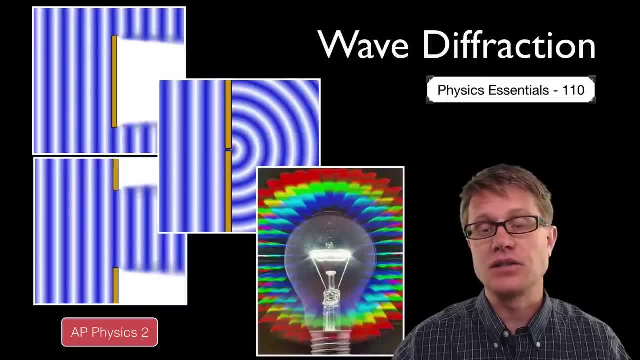 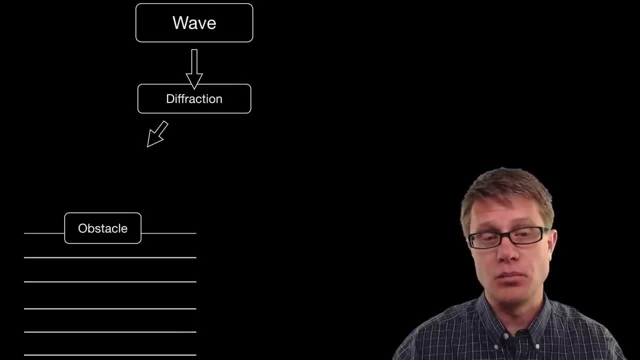 we can actually diffract light and break it into its different constituent parts, And so wave diffraction occurs when we have either an obstacle or we have some kind of an opening, And as the waves hit the obstacle they will bend slightly around it. So an obstacle can. 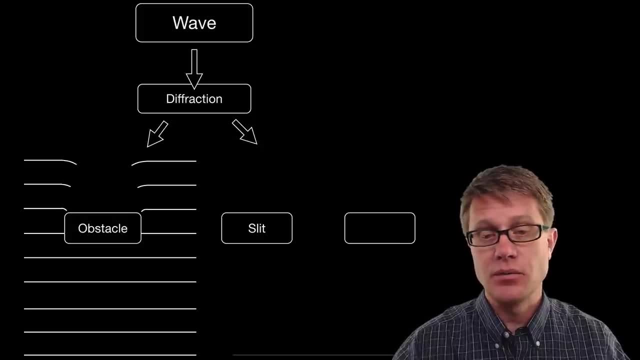 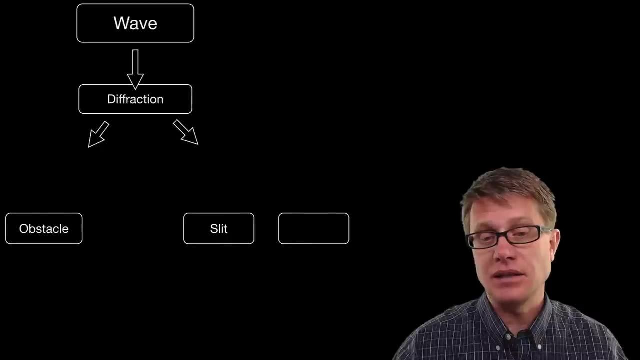 diffract waves and also a slit. So as it moves through we are going to see a slight amount of diffraction as well. It is bending around that opening. But what happens? if we take that slit and we make it the size of lambda, the size of the wavelength, what you get is true diffraction. that is going. 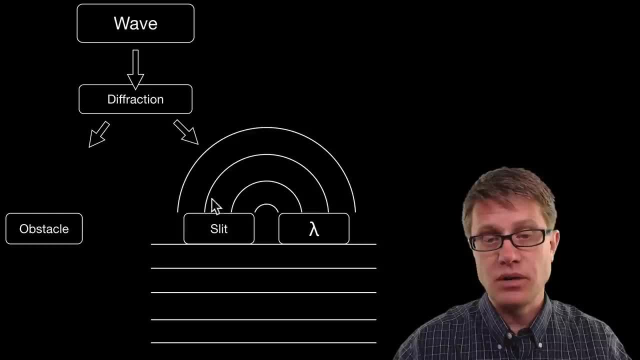 to look like that. So what is an example of this? Let's say that you are here and somebody is talking in another room. Can you hear them talking? Yeah, And that is because the sound waves are relatively large. As they move through the door, they are going to be diffracting. 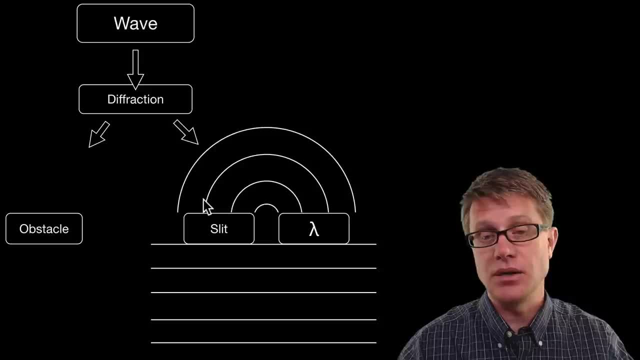 So you can hear what they are saying. It might not be super loud, but you can still hear it. Now, can you see them around the corner if you are in a different room? No, Even though light can be diffracted. look at our opening. Our opening is so big compared to the wavelength. 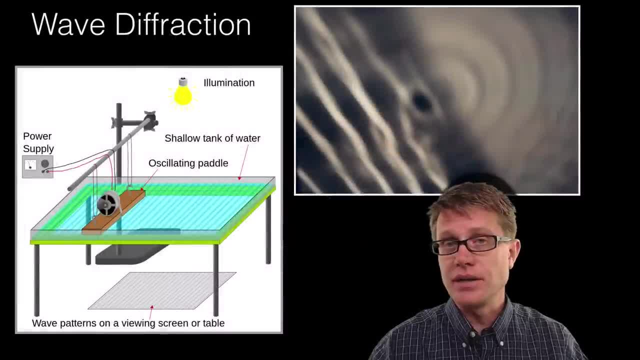 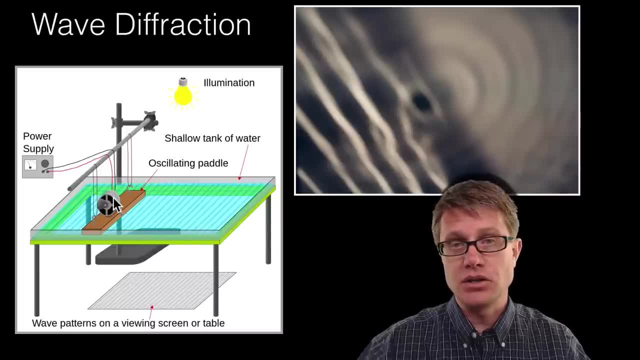 of the light that it is not bending around that corner. A good way to see wave diffraction is to use a ripple tank, And so what you do is put a table that has water in it. You then have a motor that just goes up and down, And as it goes up and down, this board oscillates. 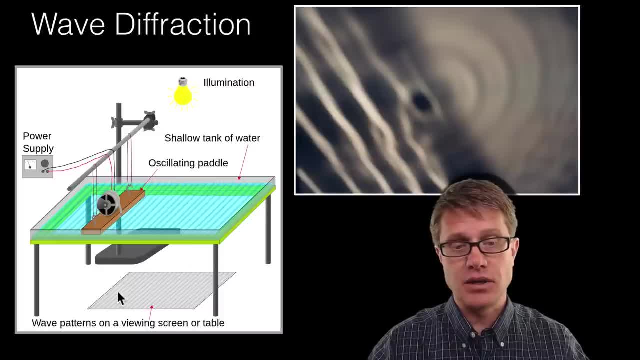 And that creates waves that move out. You can shine light through it and then we can take a picture on the bottom, And so this is what it would look like, where you have these waves that are being created, And then you could see this gap. So they are moving. 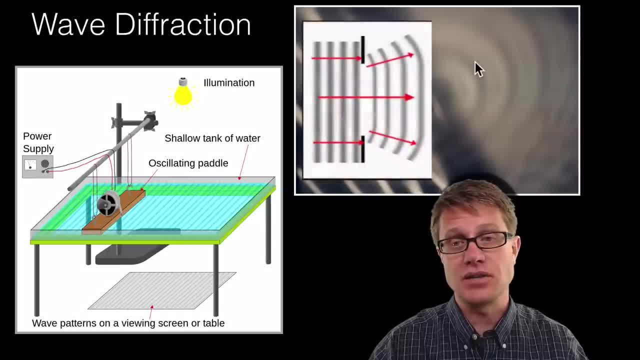 right through this gap right here, and so you see diffraction on the other side. Now the size of that gap is important. If you have a gap that is really really large in relation to the wavelength, small diffraction. But if we decrease it to around the size of the, 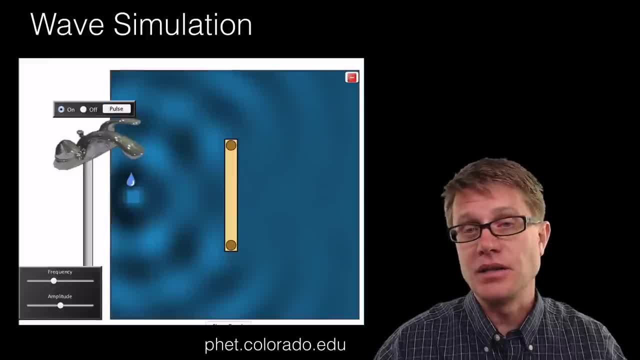 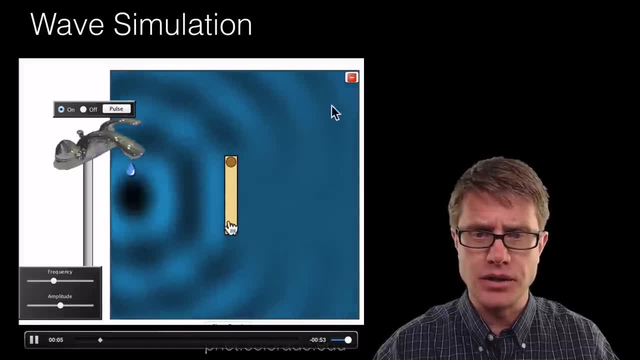 wavelength, then we are going to get true diffraction. Here is a little PHET simulation of that. So we are generating some waves on the left side- water waves- and we are seeing diffraction over here. You can see it bend around, But watch what happens as we make that smaller.